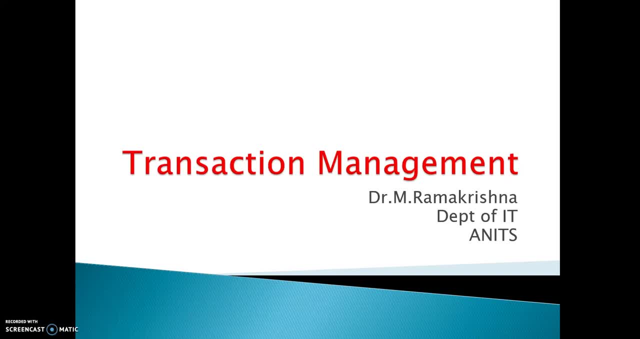 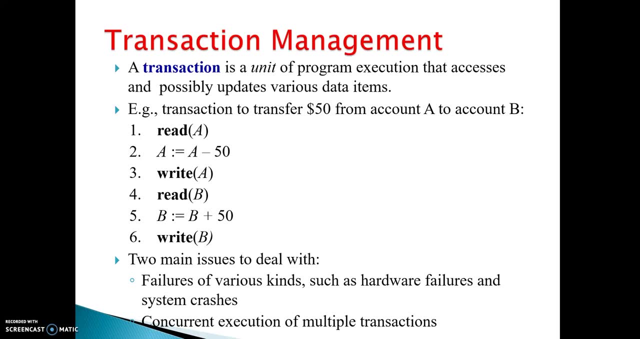 How to manage the transactions properly with a consistent manner of database. Exactly we are talking about in the transaction management. Let us see here what exactly a transaction is. first, A transaction is a unit of program execution that accesses and possible updates various data items. Let us see we can transfer a funds from one account to another account As an example of a transaction. If you do this type of transactions, it should be made. 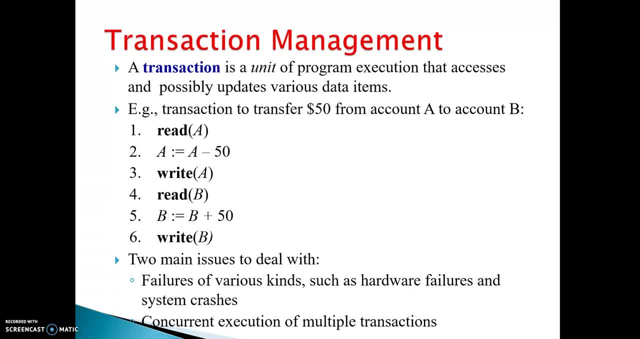 managed properly. Otherwise it leads to the inconsistency of database, which is very costly affair. So in this example of a transaction, we transfer $50 from account A to account B. Let us a simple transaction in this case. Here we look at there are six steps this transaction has been happening and each step we simply called as an instruction. In this case, look at a first step. 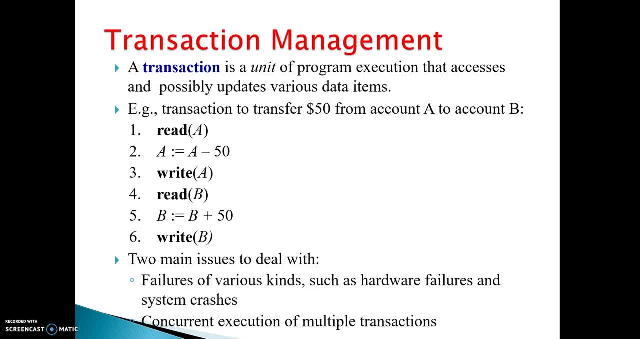 we did A. It means read the amount in the account A. and the second instruction is talking about deduct $50 from the account A. Once deducted from A, that remaining can be stored. this into the memory that, in the place of write A, Once it writes it read the B accounts information and add $50 into B has a fifth instruction. 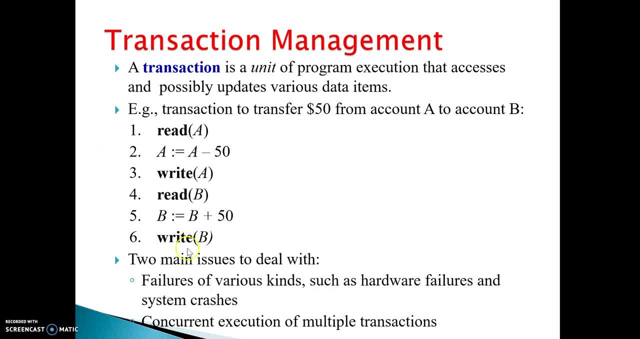 Here b is equal to b plus 50. and last, we can write this information in permanently into the b account. So these six steps is simple. we called it as in a transaction: transfer of funds of 50 dollar from account a to account b. right, This transaction has been happening perfectly, right. 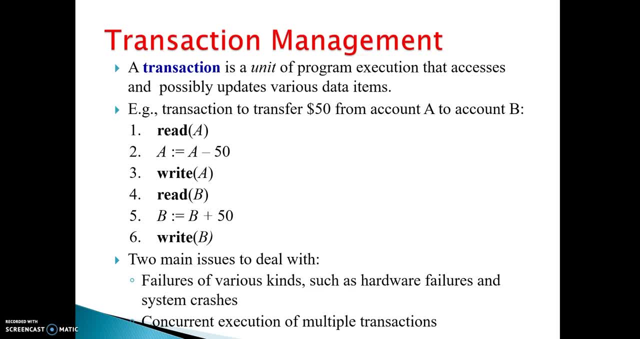 nothing is a problem, but in our scenario there may be a. different types of issues are came into a picture. Let us see while happening, while transferring this funds from a to b. in between, there is chance of failures. It might be various failures may be reason. it may be hardware failures. 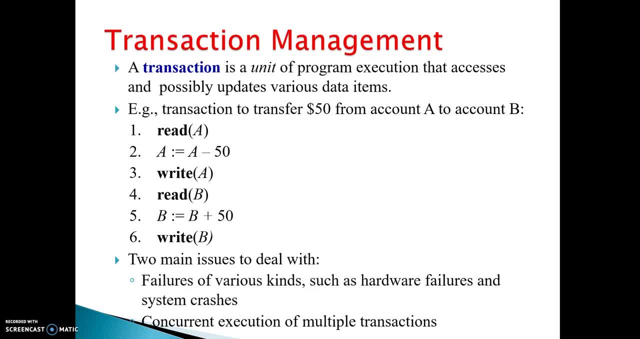 system crashes, software failures may be other different reasons to failure. this execution of transaction number one. Number two: concurrent execution of multiple transactions. Let us see now. we need to understand what is concurrent execution In every one of us. know that we need to understand what is concurrent execution In every one of us. know that we need 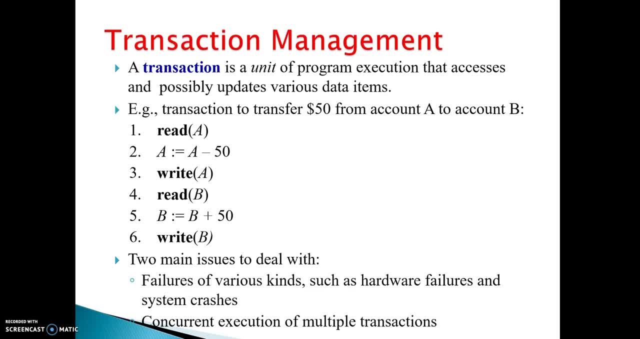 know, we are converted from batch processing into concurrent execution. We can execute more than one transaction simultaneously. It is talking about a concurrent execution, So the multiple transactions are executing concurrently. There is also a possibility of happening inconsistency in the database. So, keeping all these things, we need a proper management system to maintain of the 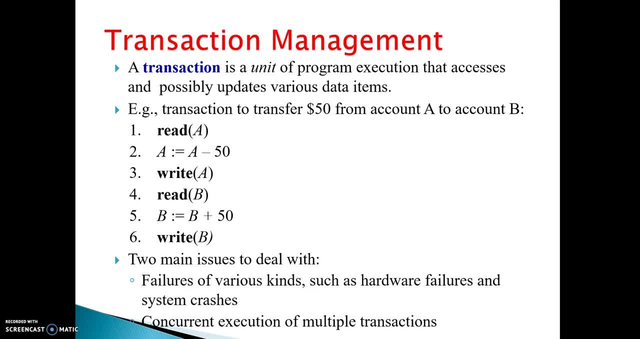 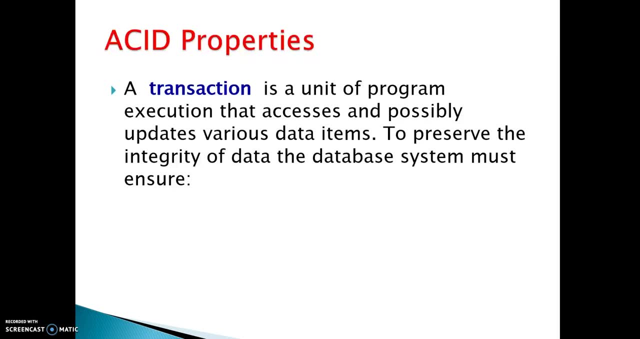 transaction execution. This is what mainly concentrate on transaction management. So now let us move. Okay, a transaction has been executing. What are main things we need to be look at? So in this point, initially preferred, there are four properties, which is very simply called as ACID properties: A, C, I, D. So, as we discussed, 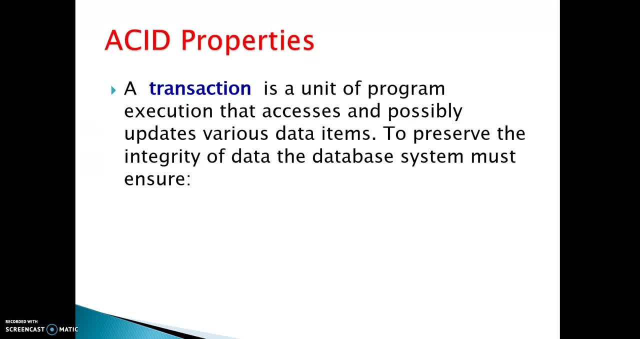 a transaction is a unit of program execution that acts and possible updates various things- data items- So there is an update in that particular data item. To preserve the integrity of the data, The database system must ensure that integrity and consistency. That's what this ACID properties are. 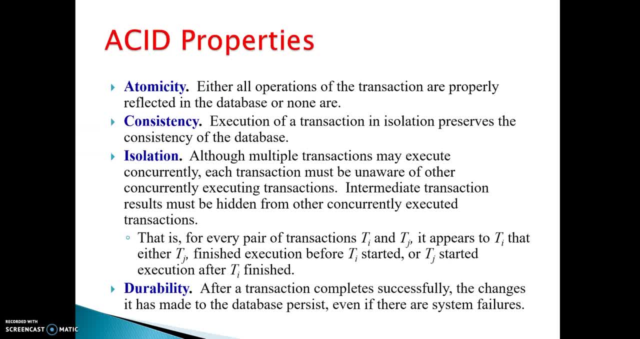 going to be look at. Let us see there are four properties with names: A means Atomicity, C means consistency, I means isolation and D means durability. there are these. these four properties are very essential and important in the transaction management to keep your database consistent. let us see the first. 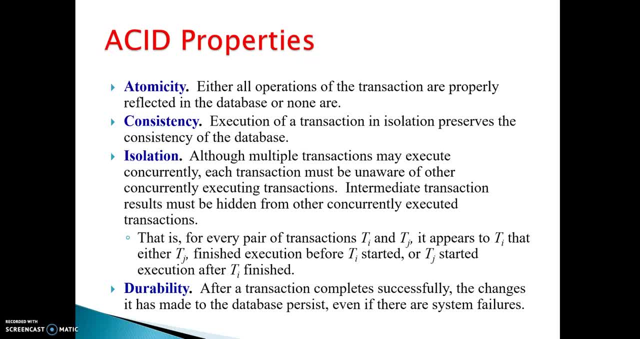 one atom city. it indicates very simply in a transaction either all the operations or the instructions that can be executed properly. reflects the database properly or not? it means in a transaction all the transactions executed properly or none of them can be executed. let us see in a simple half of: 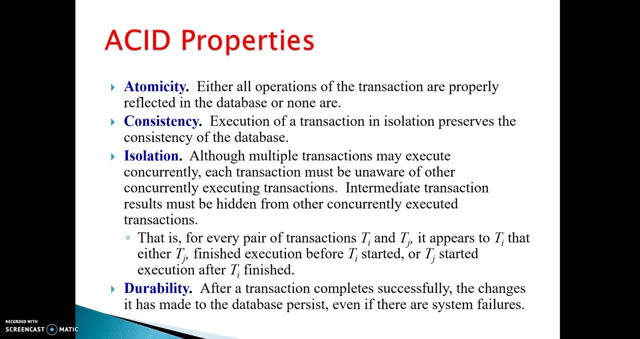 the transactions are executed. rest of the off may not be executed. let. in the case of the first transfer funds from A to B, we can deduct from a account 50 rupees. after the deduction the transaction failures. the $50 may not be added to B account. it leads to the inconsistency. so the term city is: 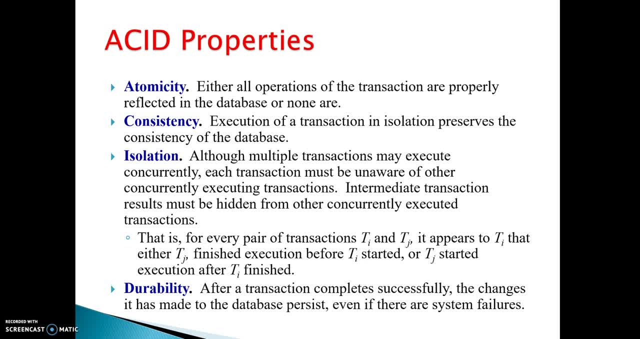 talking about either all the transactions or all the instructions are executing in a transaction perfectly or none of them- and look at consistency. the execution of transaction isolation preserves the consistency of the database. that's what. whatever the transaction you have been performed in the database, the database should be preserve its consistency. 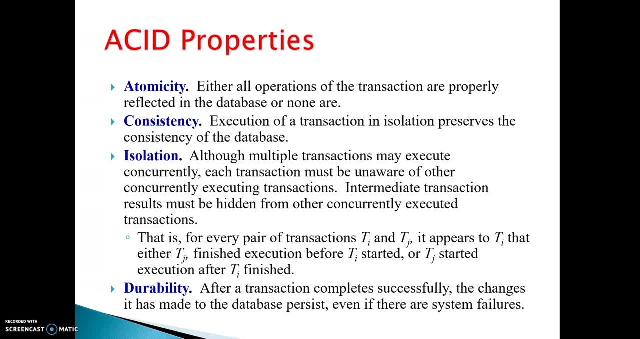 you can see that in the first example, if you have a transaction in the database, that is talking about consistency and isolation. as for in the second property- second thing we discussed about a- multiple transactions may execute concurrently because we are converted from batch processing into concurrent execution. the reason being: we transferred from batch processing to 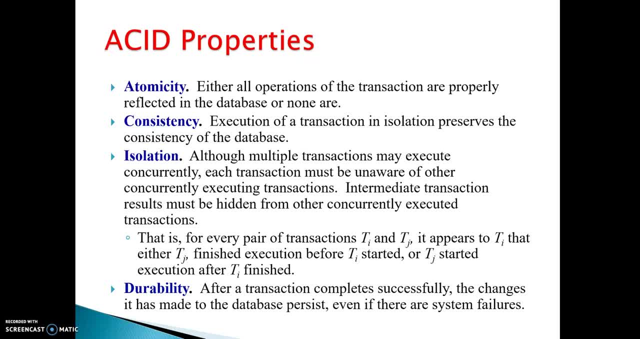 concurrent execution to improve the throughput and response time. so in this each transaction must be unaware of other concurrent execution of transaction. in this case, intermediate transaction result must be hidden from other concurrent executed transactions, otherwise it again leads to the inconsistency the isolation property is looking about. the concurrent execution of transactions are going to be taking. 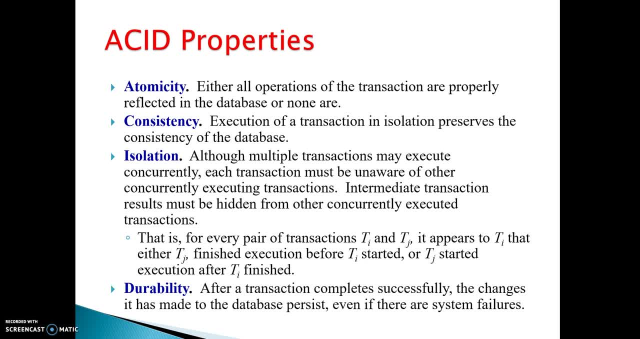 care and a durability. after transaction complete successfully, the changes it has made to the database persist even if there are system failings and the process is not good yours. so once the transaction executed correctly, that should be keep properly. the database should be stored properly in the memory. so these four properties are very much important. 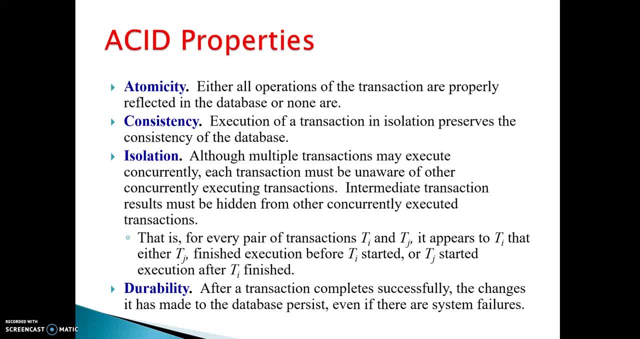 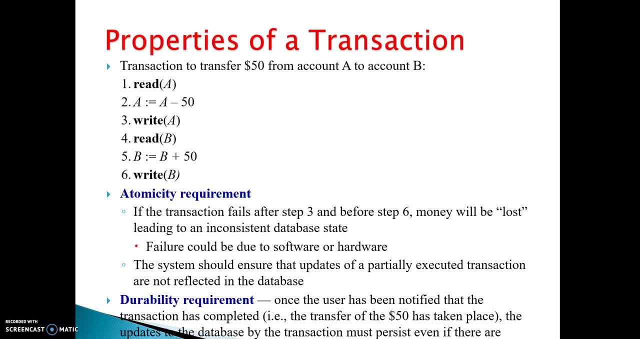 to performing a transaction management system, so to maintain these properties. so let us take a same example, what we discussed about transaction to transfer our funds from a to b, a fifty dollars in this case of atom city. if the transaction fails after step three, after step three, before step six, money will be lost. it means execute first instruction.